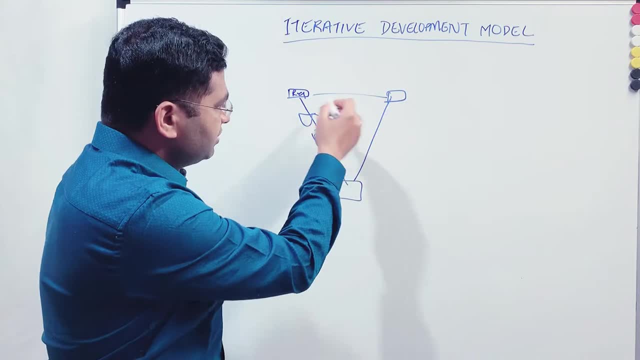 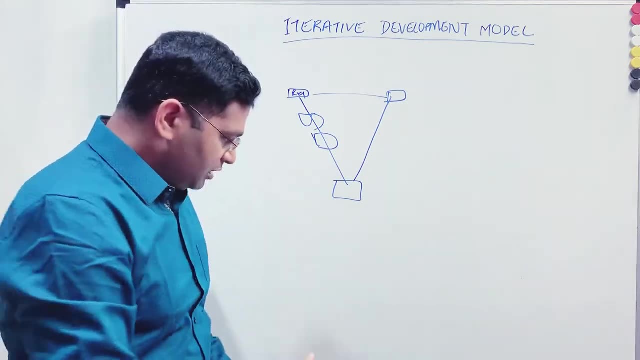 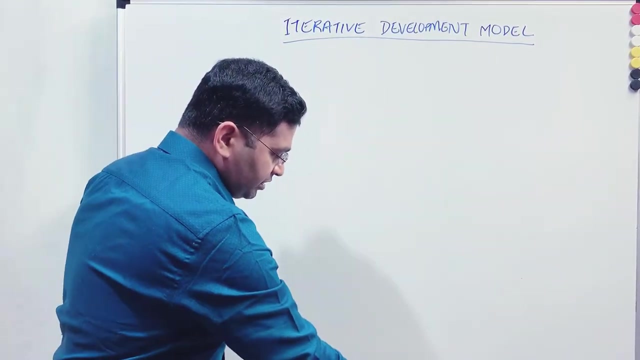 system testing, integration testing accordingly. all right, so testing was involved in each and every phase, but the duration was still lengthy. right, so the duration was still long for the v model as well as it was in the waterfall model. now, if you have a delivery in current scenario in the 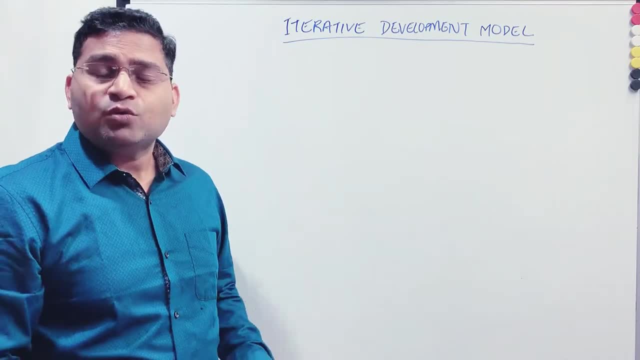 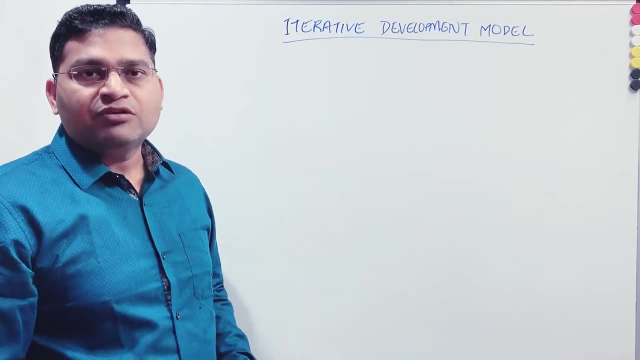 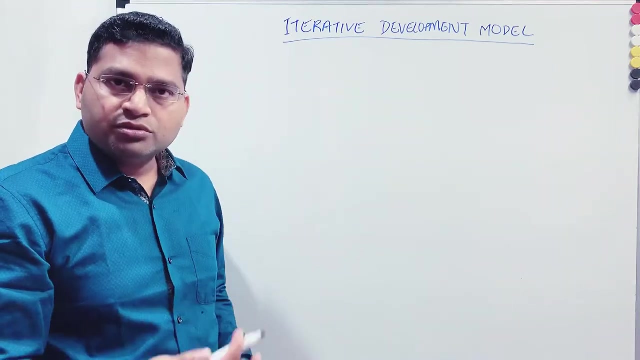 current dynamic scenario, the market conditions- you can't wait for delivering a software for you know, like two years, okay, so you have to add the value or deliver the value to the customers pretty quickly and that That is why you have to deliver software very quickly. And in order to address those issues of delivery or delayed delivery to the customer, iterative development model was introduced. 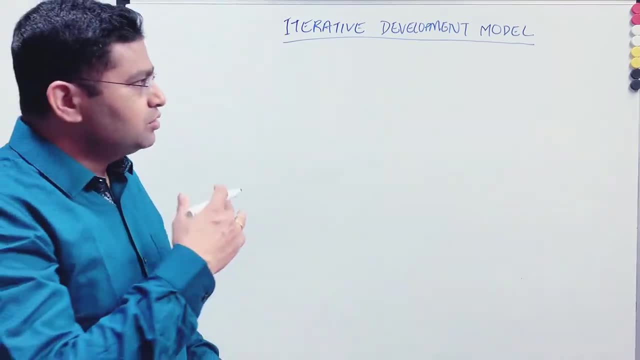 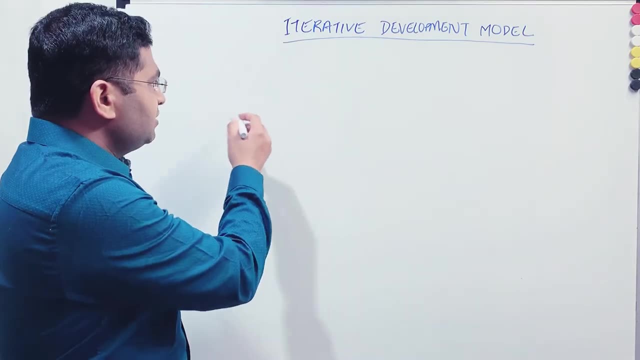 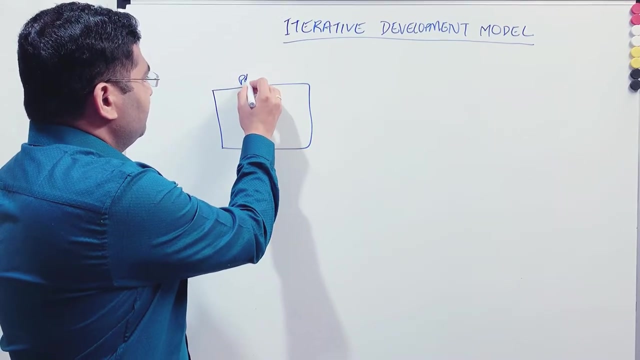 So iterative development model. what they do is you basically repeat the same cycle. So, for example, in the waterfall we had certain phases, right, So we had phases, say for example in the waterfall. So, for example, if I say phase one, right. 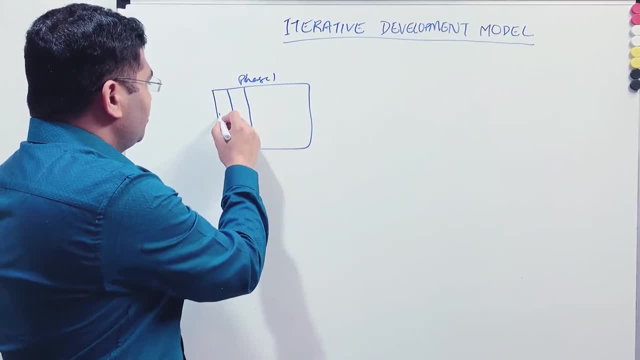 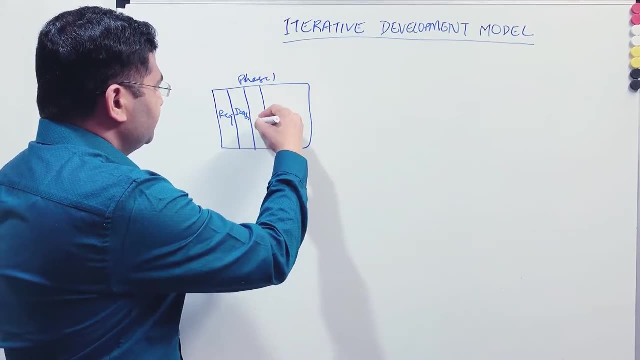 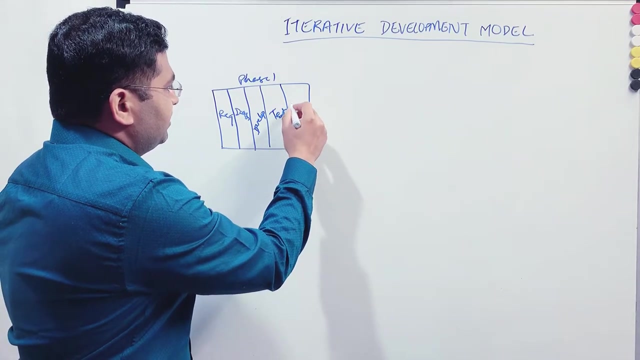 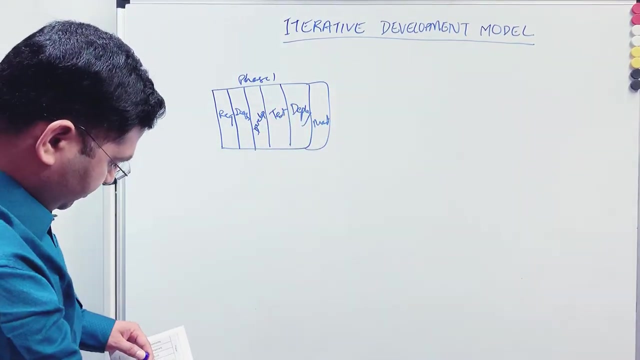 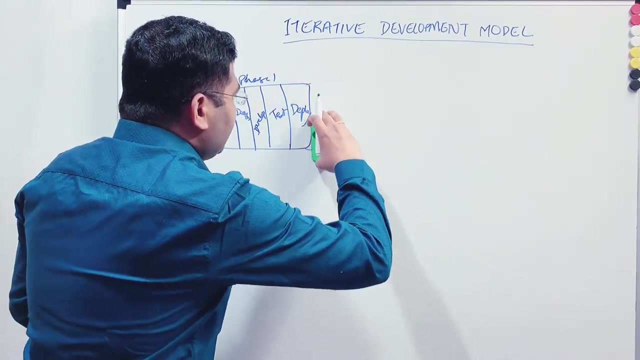 So waterfall, we had the phase of requirements. Then we have design, Then develop- OK, so develop, test and then deploy- right And then maintenance. So these were some of the phases, right? So So what happened in the iterative development approach is basically they had these phases and these phases will be repeated. 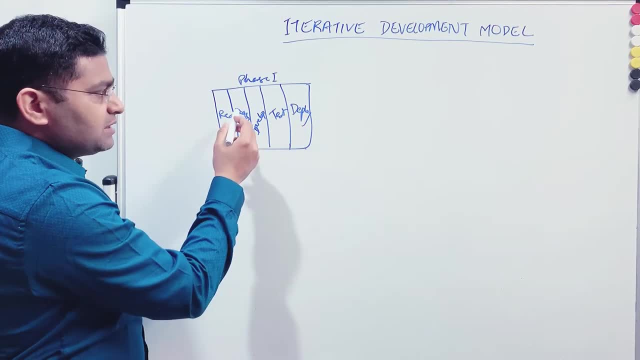 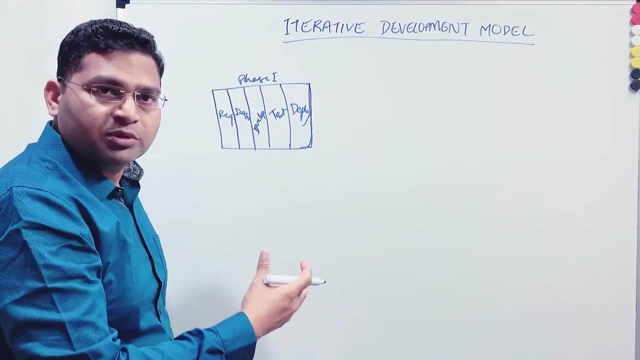 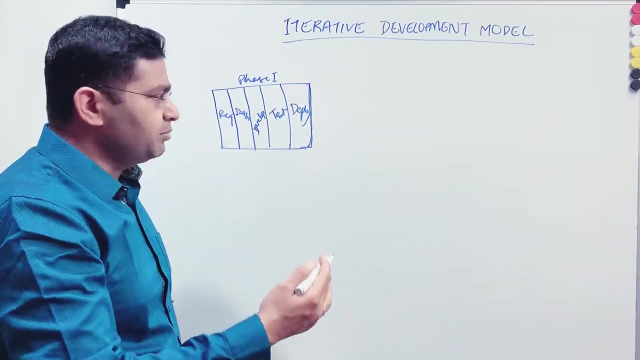 So say, for example, phase one will have the requirement then design, develop, test and deploy. So this will be sort of, you know, like a quick release of one to two months. So every four weeks to eight weeks there could be, you know, a drop of software coming or deployment happening. 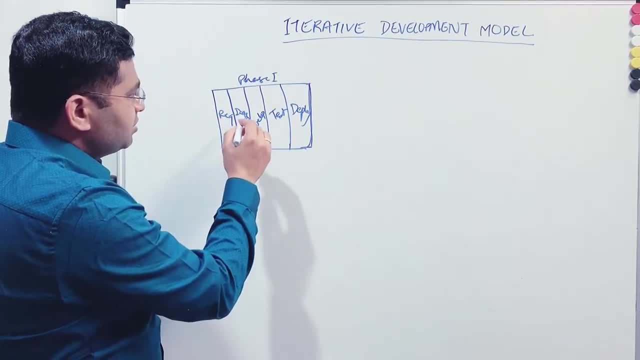 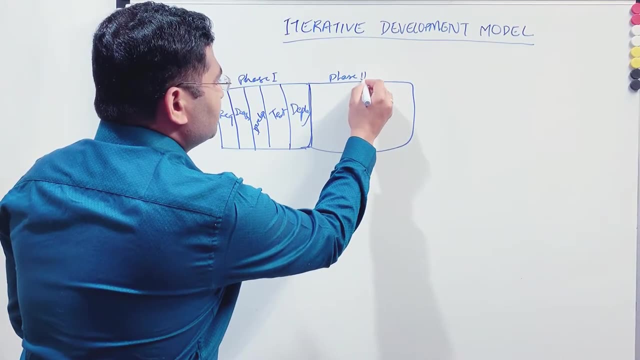 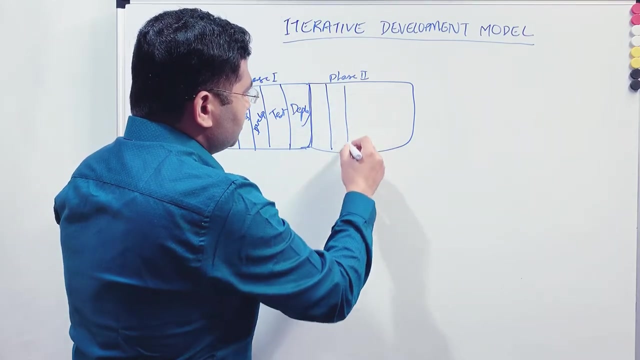 And then the same cycle. So you see: requirements, design, development, test, deploy. The same cycle keeps repeating. So there will be another phase, or a release of phase two, or a release to whatever the organization want to call it, And this whole process of requirements. 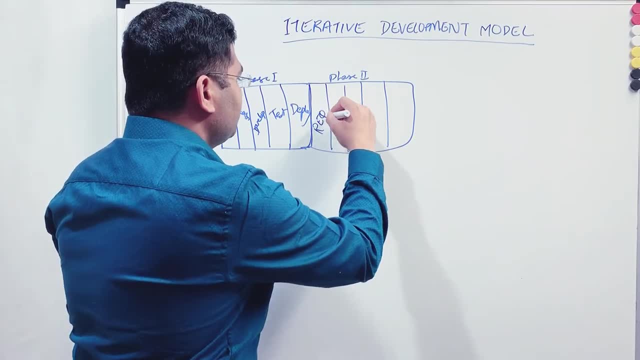 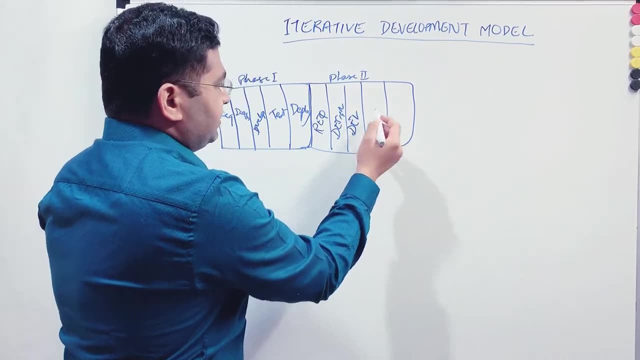 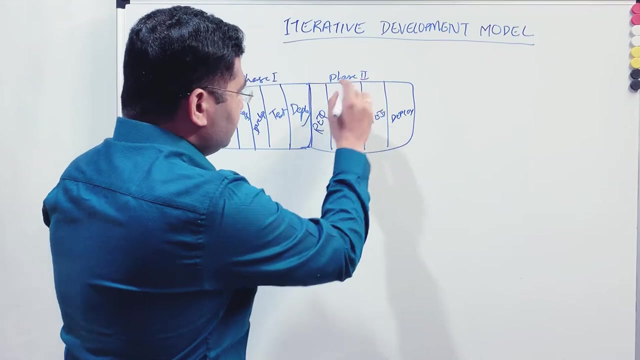 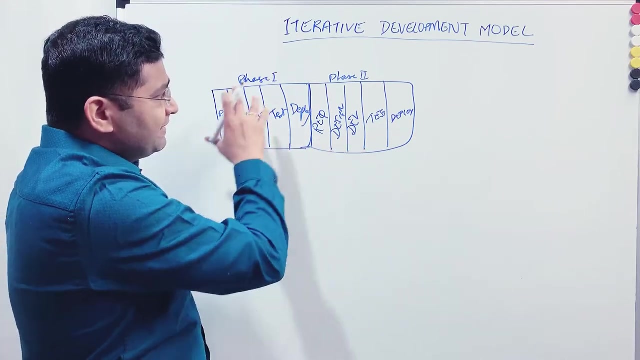 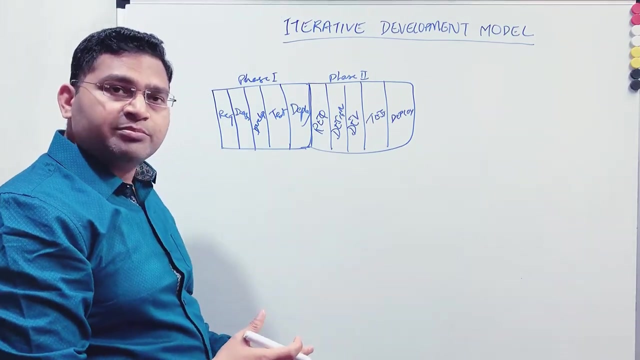 So requirement, I'll say requirement, design, develop And then, you know, test And deploy, right. So all these, all the same phases. whatever we have seen in the waterfall model, except the maintenance phase, will keep repeating in each of these iterations unless and until all the requirements that have been given by the customers are being completely built and deployed in different phases. 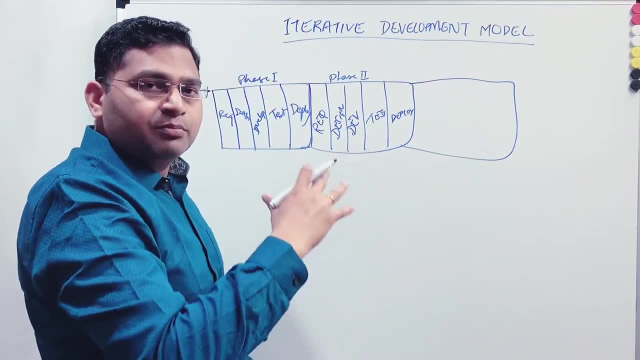 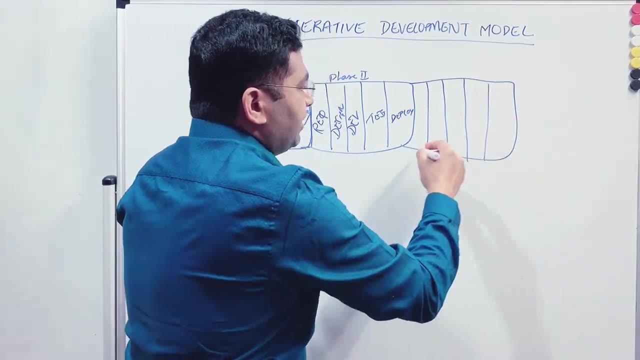 So there could be, you know, like five phases, 10 phases. So you know there, there There could be multiple phases, depending on how the complex software is and how many requirements you are trying to build. So there will be another phase, phase three, starting right. 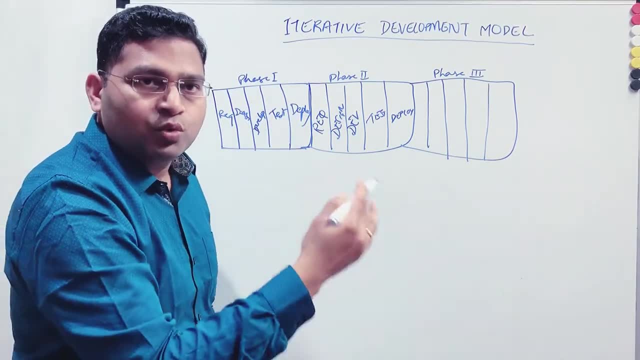 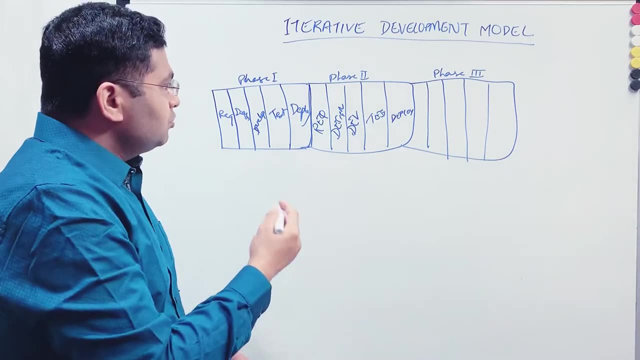 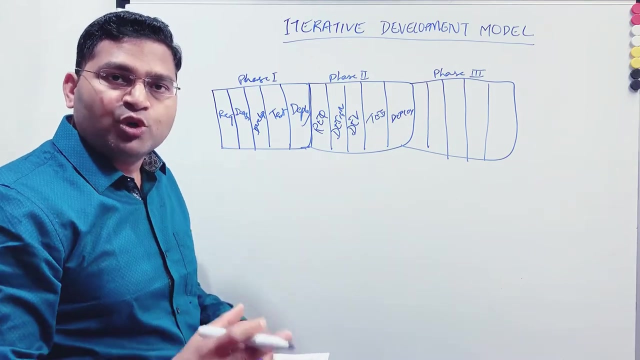 So this is how iterative development model works. Now, in iterative development model, there wasn't much change. The only change was basically to have shorter iterations or shorter cycles, And within those cycles you fit Smaller waterfall model. Okay, So here, if you see, this is one cycle or iteration. 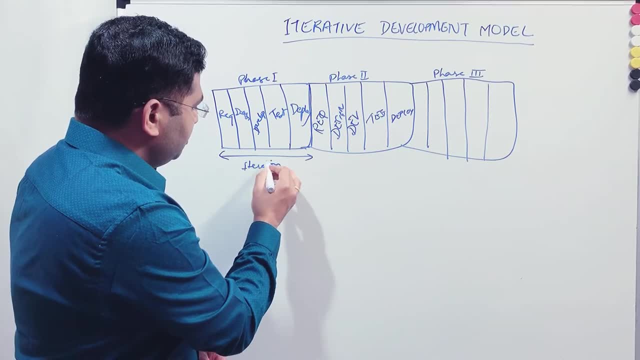 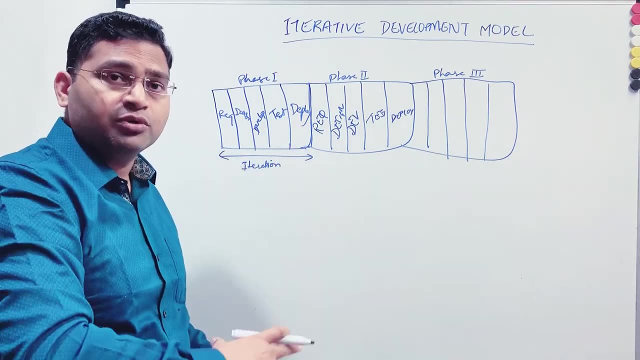 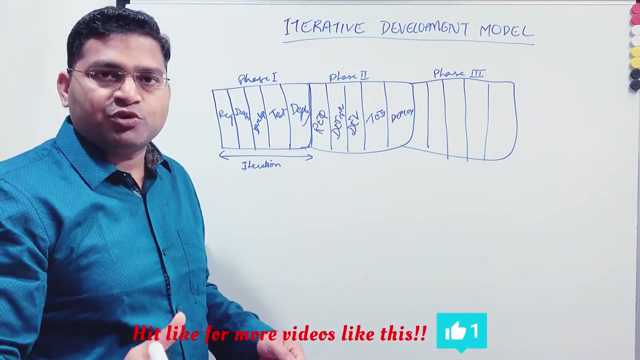 Okay, So iterative came from iteration, So, which is nothing but the duration of whatever you know, weeks or months. So it will be a shorter duration as compared to the waterfall approach. So in waterfall approach it was mostly like six months to one year. to you know, maybe it will extend up to two years as well, but in iterative it will come down to one month or two months, depending on. 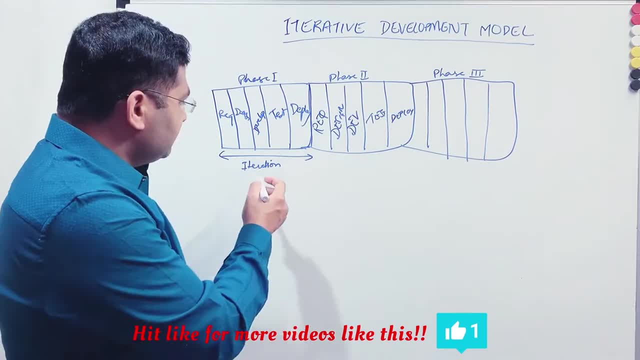 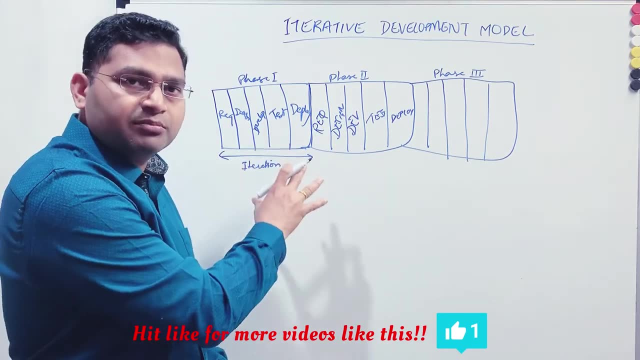 How the organization or project team wants to manage And then in the first iteration they'll pick certain features and they'll try to build some of the skeleton or the initial features. Then they'll pick another set of features in the second iteration, right, 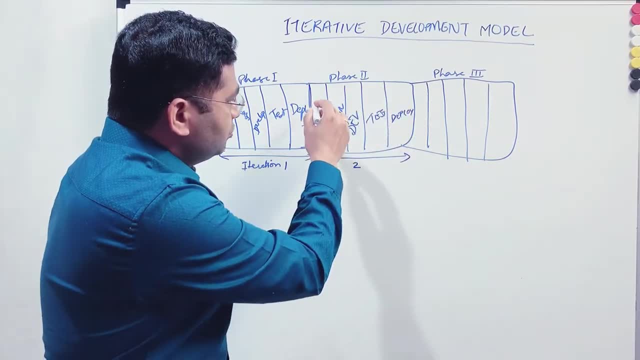 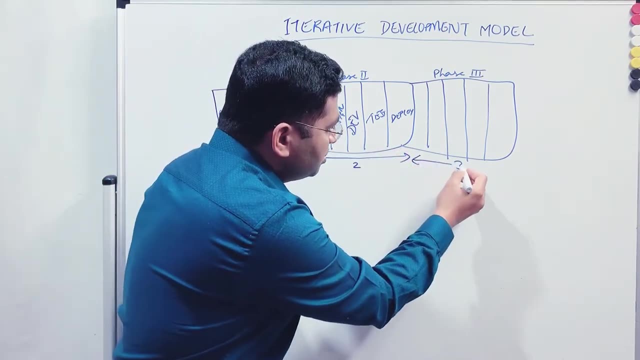 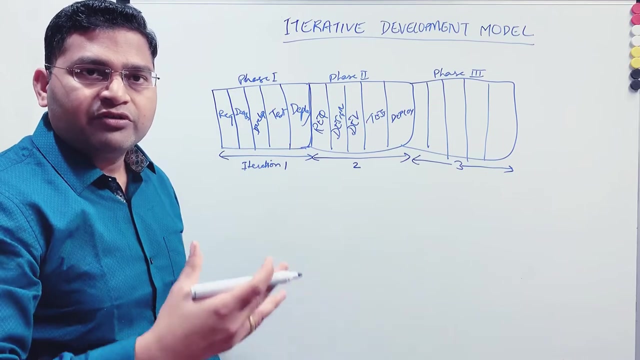 So second iteration, and they'll build. they'll do the you know requirement analysis and then design and develop, test and deploy. Similarly, this whole process will keep continuing like that. Okay, Now let's take Take an example of how um the software will be built incrementally or basically with the iterative development approach. 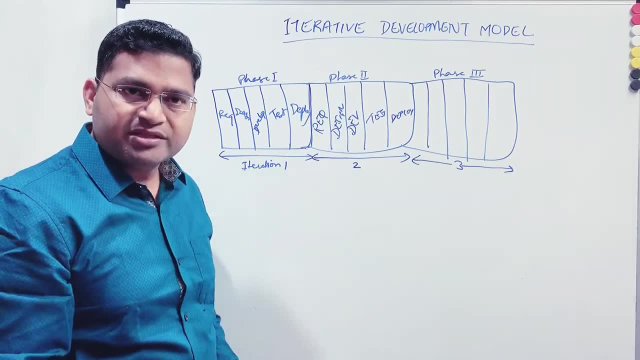 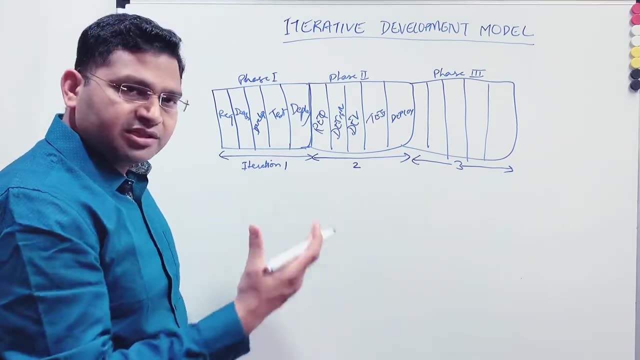 I'll say, for example, you want to build a application, um e-commerce application, which has the login functionality right. So, for example, in the iteration one, what team might do is they will say: in first iteration we'll build the login page, right. 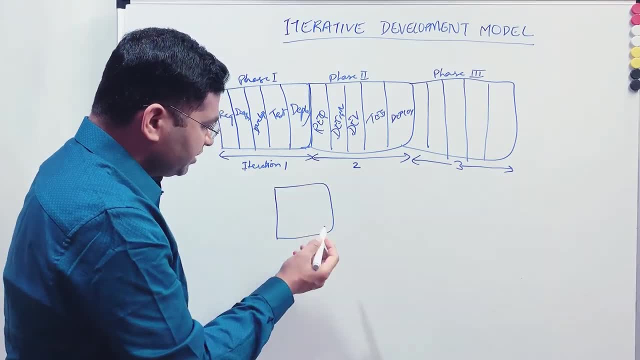 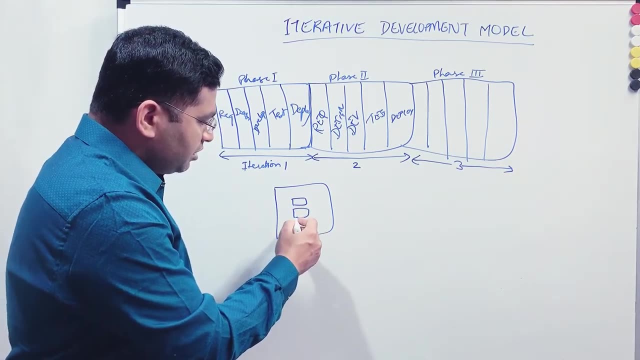 So we'll build a skeleton. So we'll have a login page, Okay, And on the login page We'll Just Have the user name and password field, Okay, And the login button. So that will be built in the first iteration. 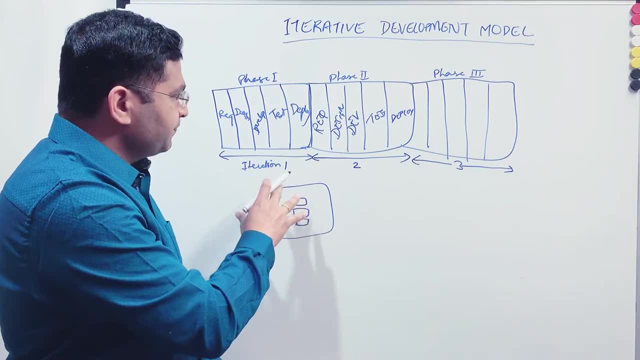 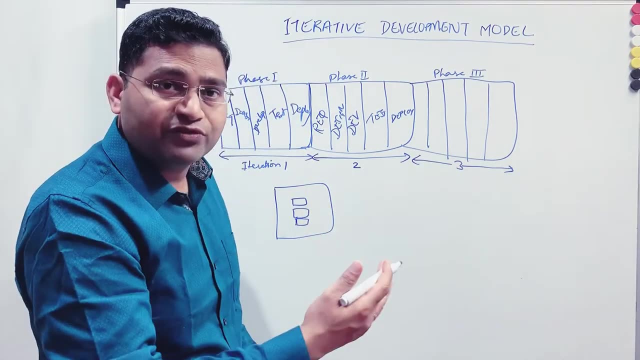 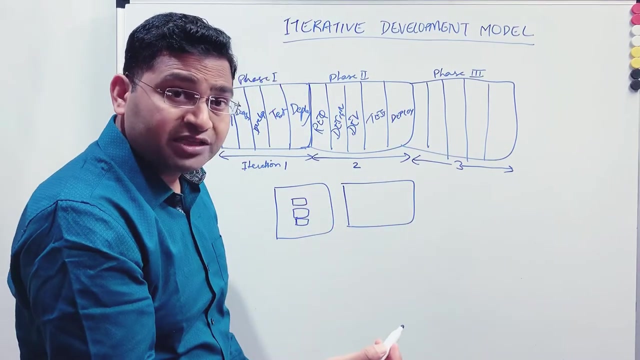 So all of this will be built, tested and deployed. Okay, Um then? um, you know, after this, they want to add more features, right, Or more requirements. So the next, what they'll do is they might add, you know they, they will beautify the page. 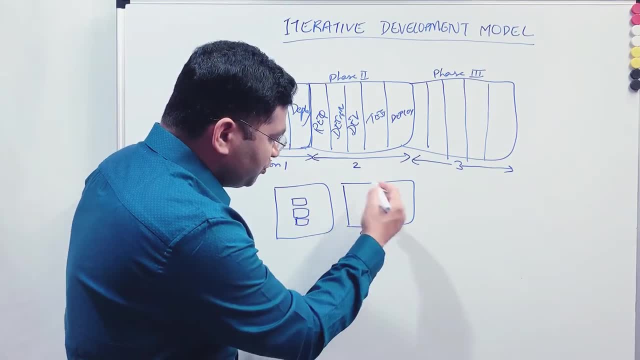 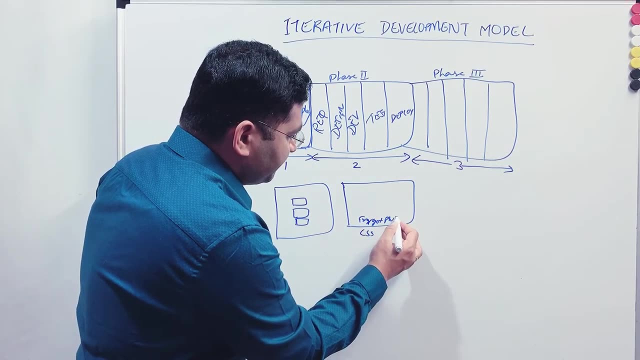 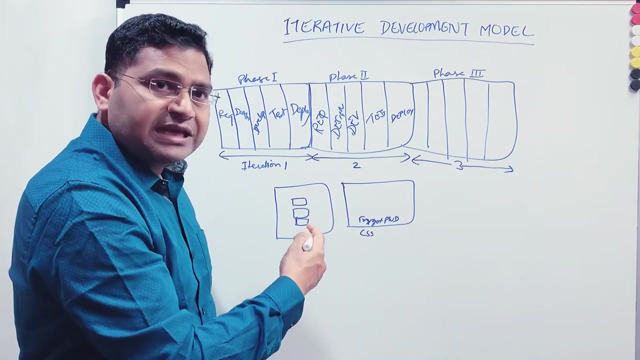 So they'll, uh, add, you know, more CSS to beautify the page, And then they might add, Forgot so Forgot- password functionality in the next iteration, Okay, Or in the next next phase. So this is how they'll keep incrementally adding more functionality in the iterations, in the iterative development model. 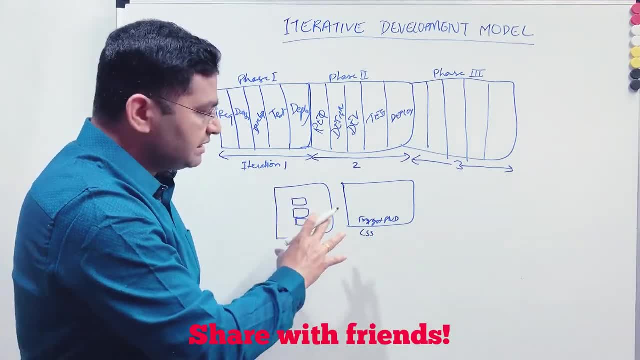 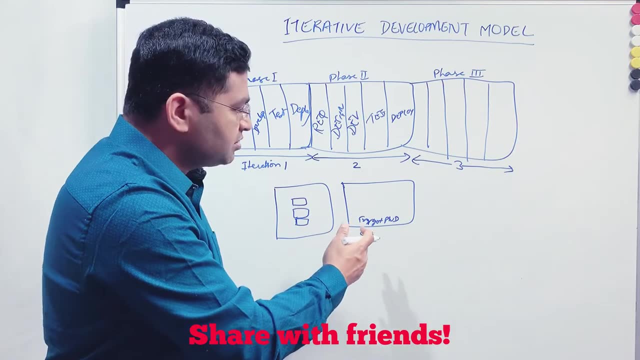 So in the first phase there'll be- in the first phase they'll do- some features. in the next phase They'll add more features like Forgot password, you know, uh Forgot username. So all those features might be added. So all those features might be available in the next phase. 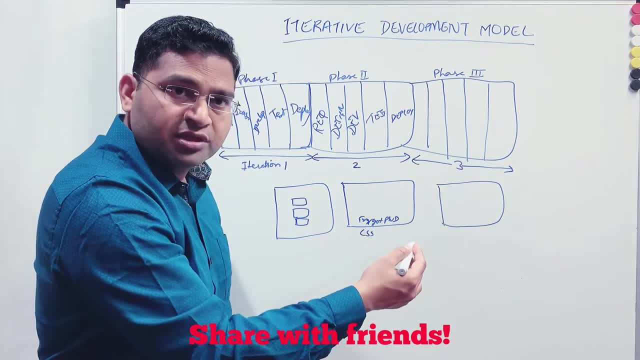 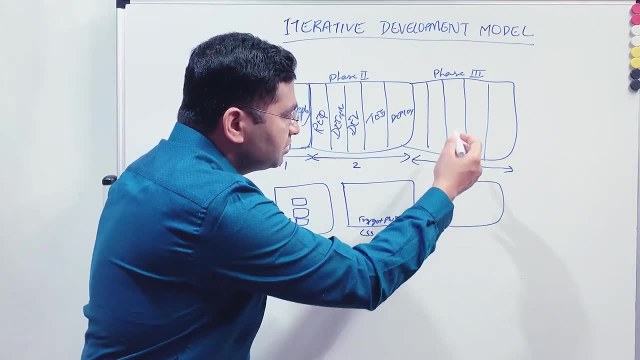 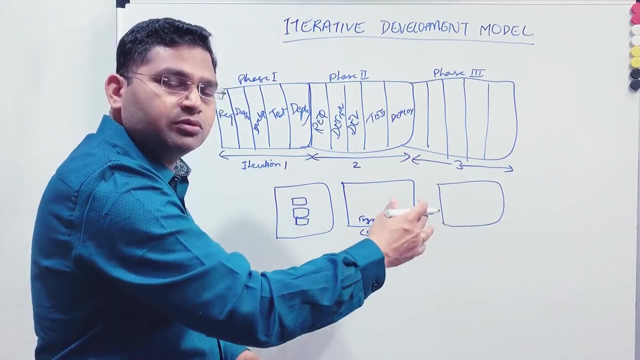 Then they in the third phase. then they might pick more features. So for example, signing up with the Google, signing up with Facebook account. So those features can come in third phase. But you can see, the advantage here is that instead of waiting for two years to get the whole you know release or the software, you can get the release very quickly. 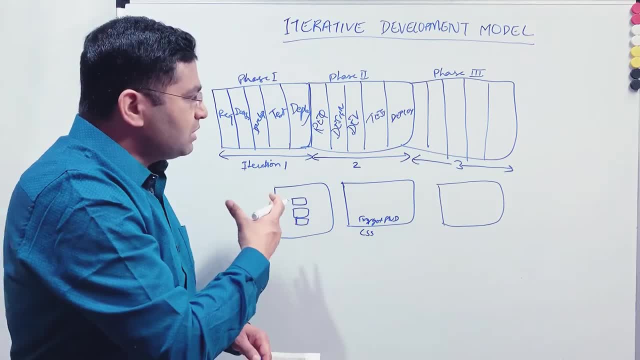 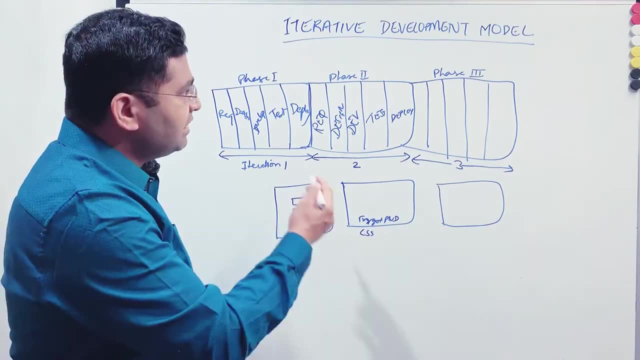 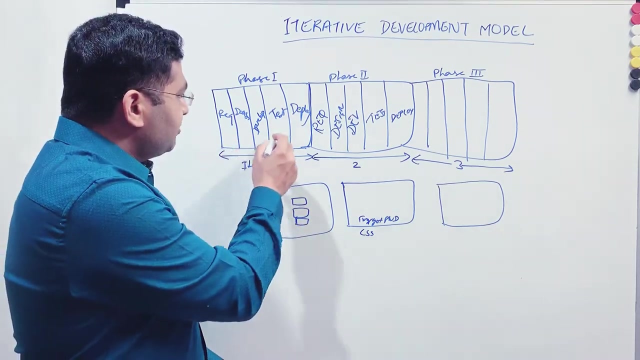 So there is something working available for the customer to have a look how the implementation has happened Okay, And whether it is meeting the customer's requirement, right. So that was the advantage of iterative development model, But the disadvantage is, again, it didn't address that phased approach, right. 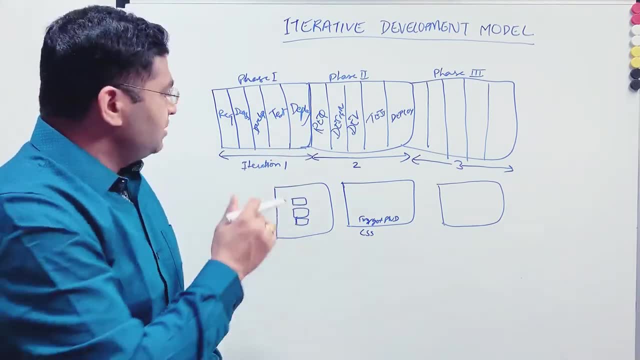 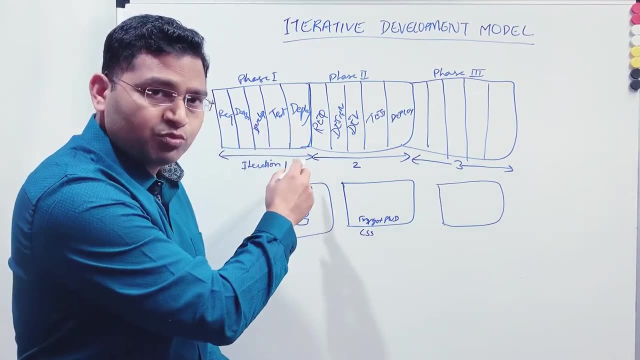 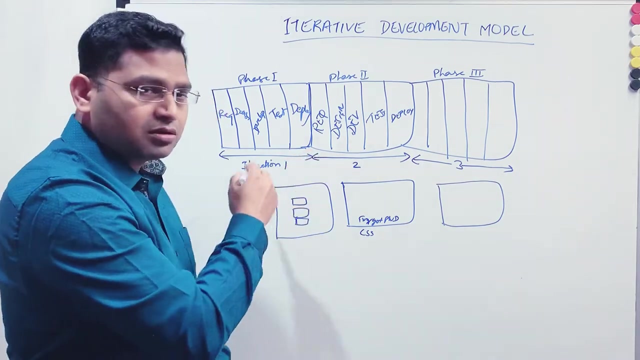 Even though the cycle is still short, but there is still phased approach. requirement need to be frozen, Then design will start, then development will start, test will start and then deployment will happen. Right, So phased approach is still there, but because cycle are reduced or there are more cycles, so there is still a lot. 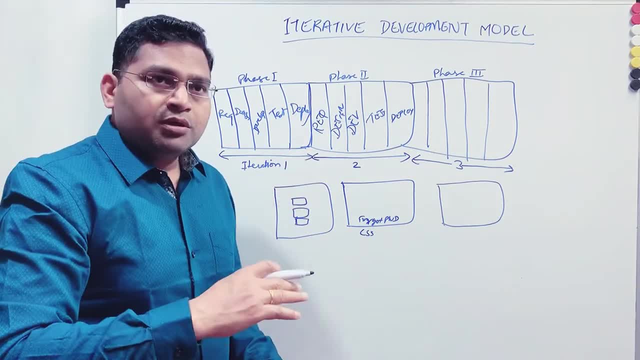 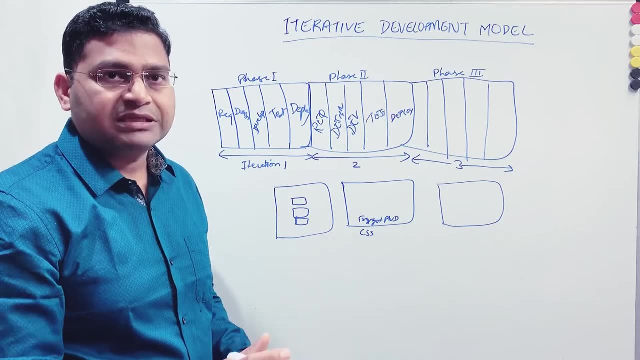 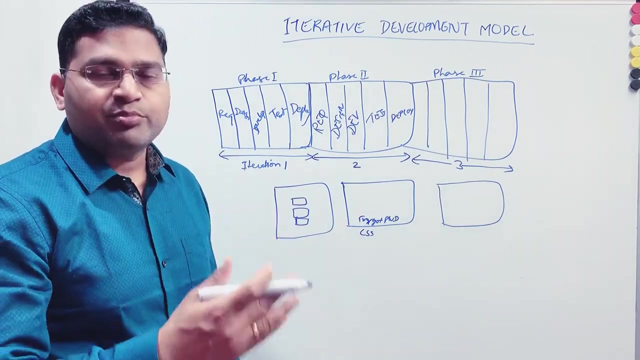 A better you know feedback loop in there. Now, agile is one you know development approach, very recent development approach, which is basically scrum, And agile is also, or it also follows, iterative approach right. So there are sprints and then within sprints you develop small features. 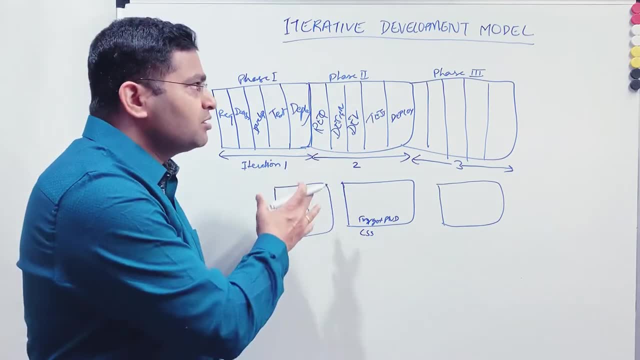 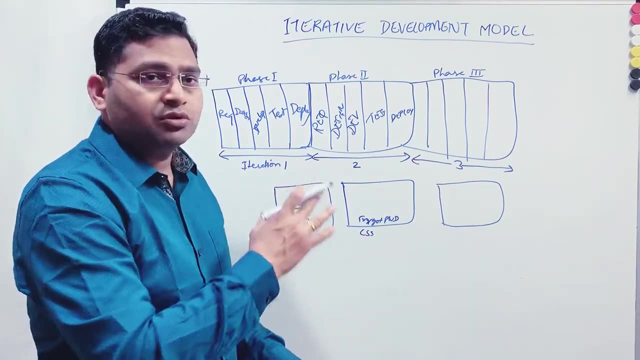 But you shouldn't confuse that. agile is exactly similar to what iterative development model is. Agile Is a lot more as compared to iterative development model. So it is similar, but it is not same to iterative development model. Please note that right. 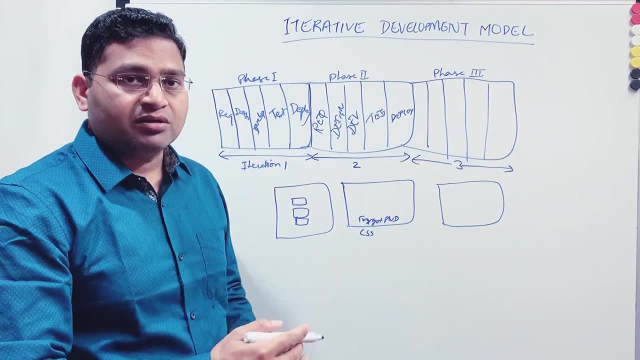 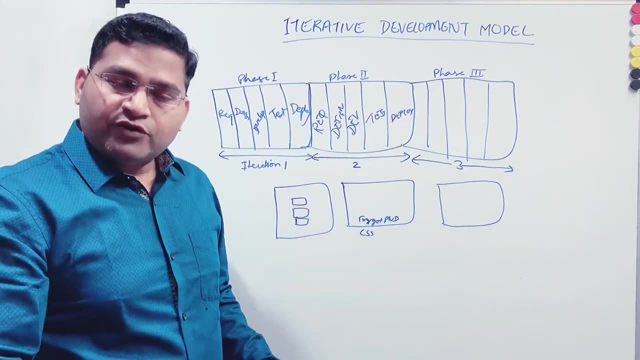 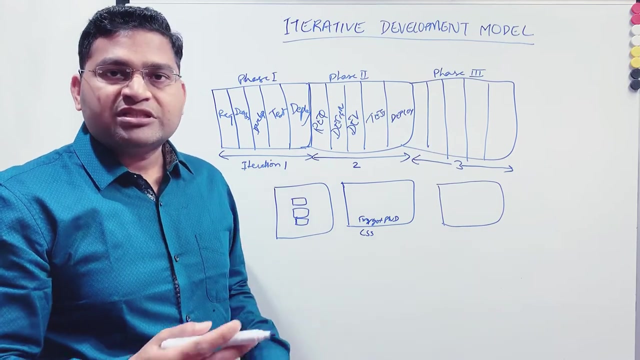 So do not get confused that agile or extreme programming they are, you know, similar or exactly same as iterative development model. So they follow that cadence. They follow that you know smaller iterations, but there is a lot more in agile which I'll explain. 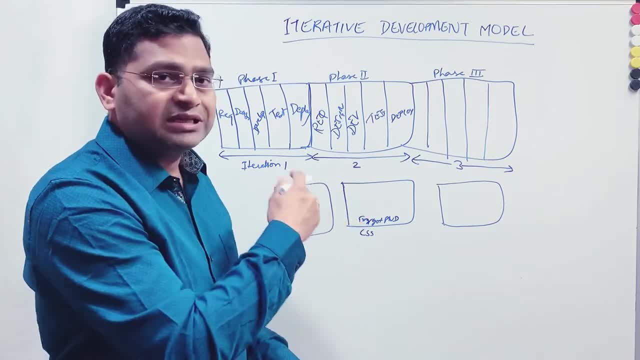 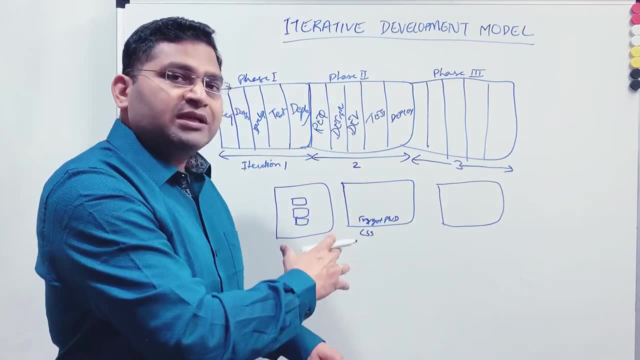 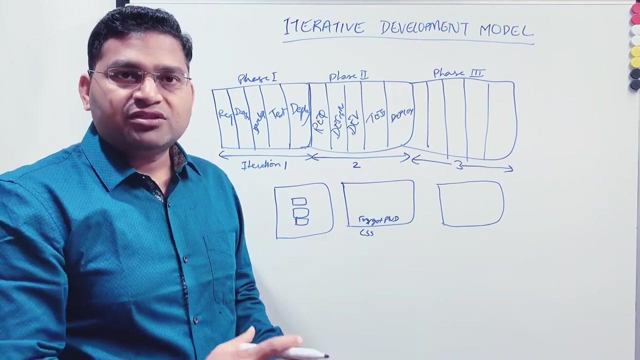 In later tutorials as compared to iterative development model. So in agile a lot more drawbacks that were there in waterfall approach in V model, in iterative model as well They were being addressed and it's totally a different. you know mindset and values that needs to be followed when you are following agile methodology or any agile development approach like scrum. 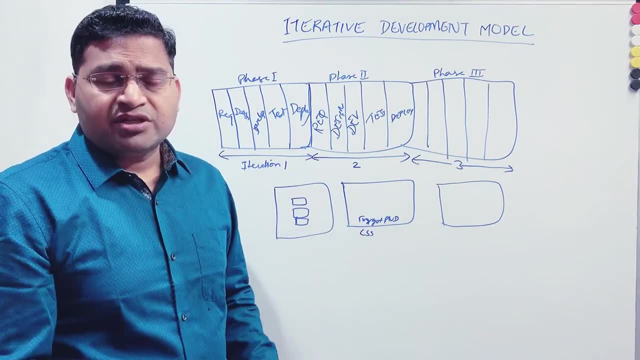 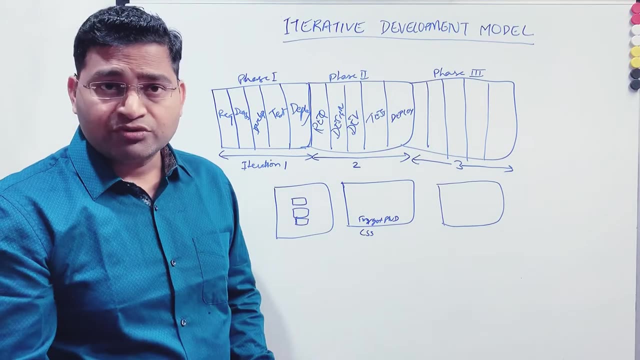 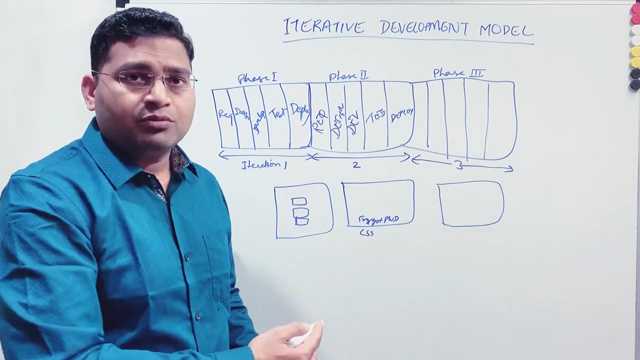 So that is all for this particular tutorial about iterative development model. Hope it was helpful And clear and will be helpful for you in your interviews. If you are going for an interview and somebody asks for what is iterative development model, whether it's similar to agile or what is the similarity. 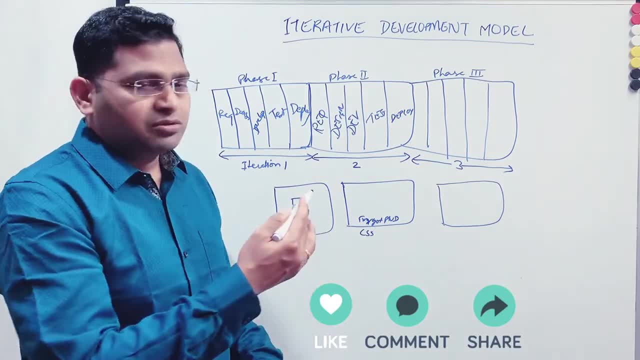 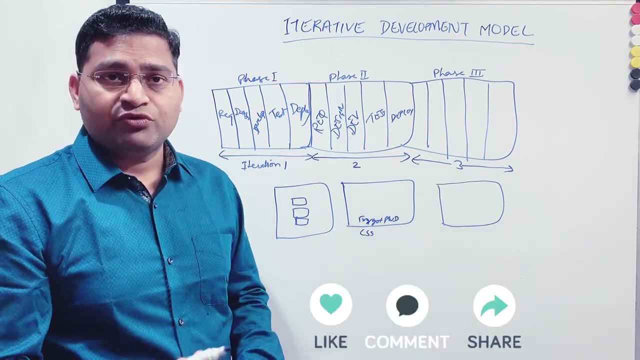 And so all those things you can answer to the interviewer, and even if you're working in any project, it will be really helpful to know all these basics before you can actually become a really good tester. So that's all for this tutorial. Please do share and subscribe. And thank you for watching.